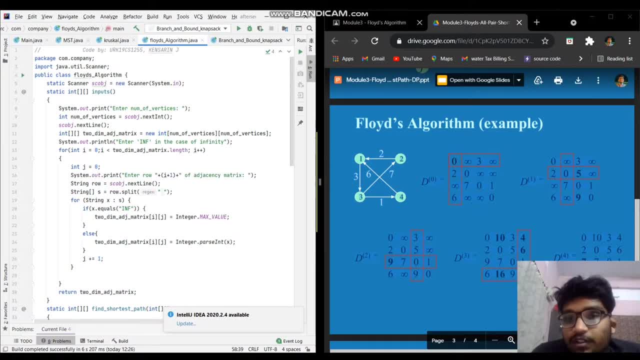 we can go from 2 to 1, but we cannot come from 1 to 2.. Fine, That is the case. we have given infinity there. We consider case where infinity is at 1 comma 4, so that also indicates a same can not go from one to four And also 2 to 3,. 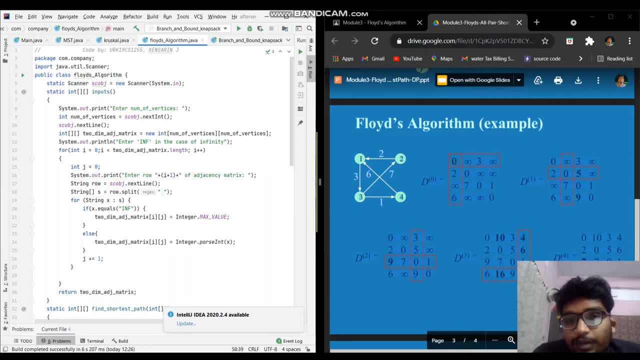 yes, 2 to 3, the direction is from 3 to 2, right, So in that case, those are the cases where we give infinity in the cost matrix, So that is, that's the thing I have given here- enter infinity in inf in the case of infinity. so in java we cannot have the infinity symbol, right? 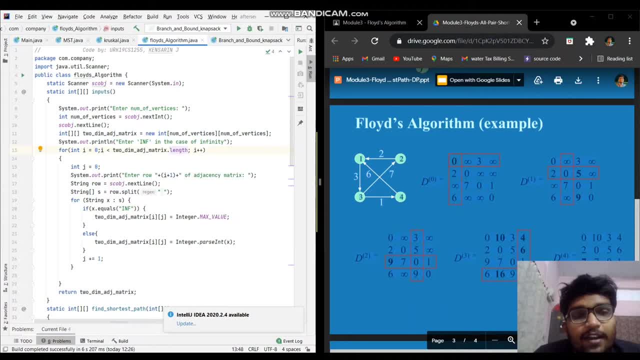 so in that place we can just have, uh, the integer dot max value in that case. fine, so we are probably easier to enter some string value as inf. so if the user enters that, so we're going to fill that entry with integer dot max value when uh. after that we are going to return the cost matrix. 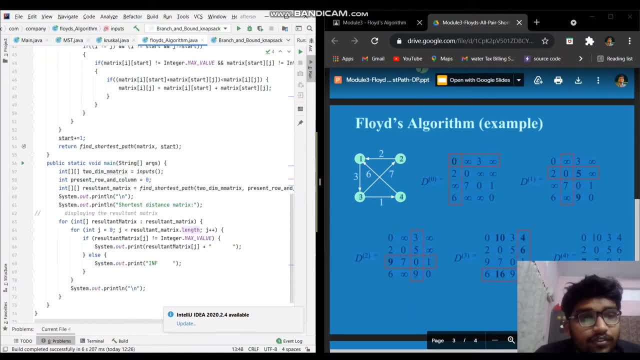 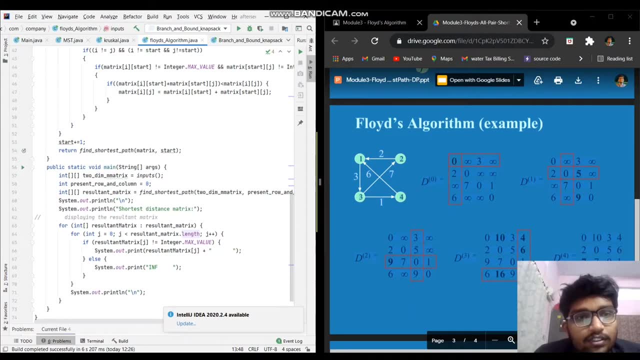 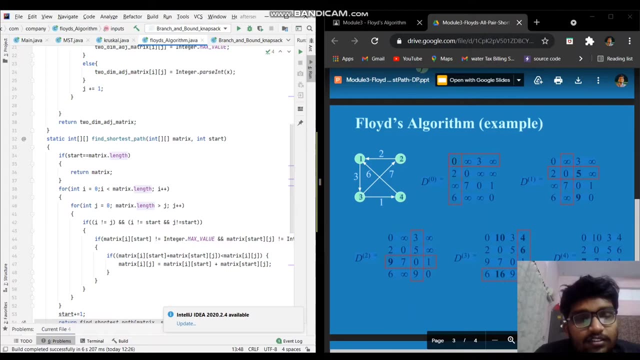 fine, uh, to the input function below, where we have called so here, and after that, uh, we have added the function called find shortest path. so now let's see the function here: find shortest path. and uh, the input for this function is matrix and the start so this matrix is nothing but cost. 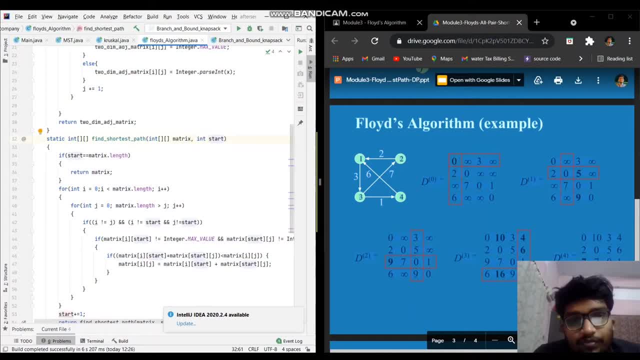 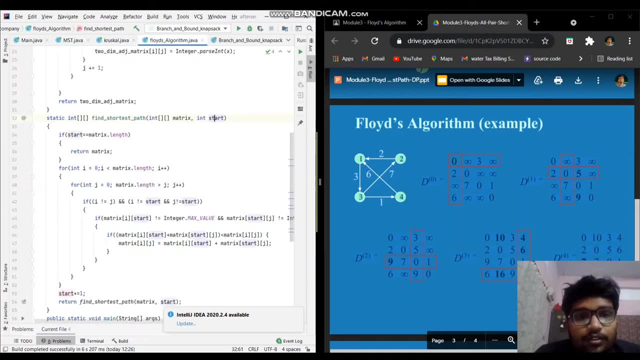 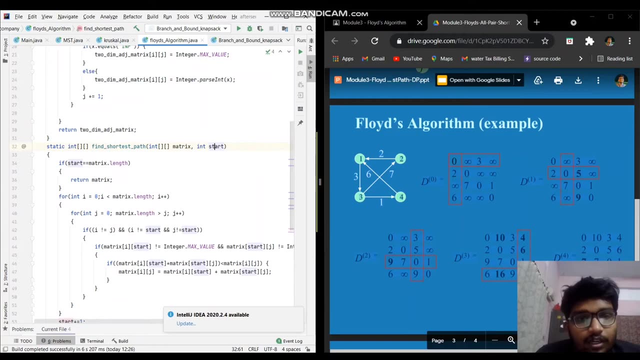 matrix and start is nothing but uh, that is zero. so in this um for finding shortest path between any pair of vertices, we're going to uh, we're going to select any uh, any row and column. so first we'll start with uh- zero. so this uh, we are passing zero to this variable. 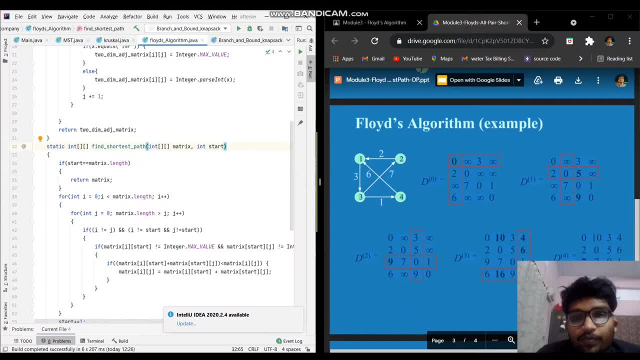 it's fine. so we are going to select row and column as zero, so the first row and the first column will be selected and, uh, we're going to check, for example, if you have to go from two to one. sorry, uh, this, this entry is uh two and two, right, so consider this infinity, which is: 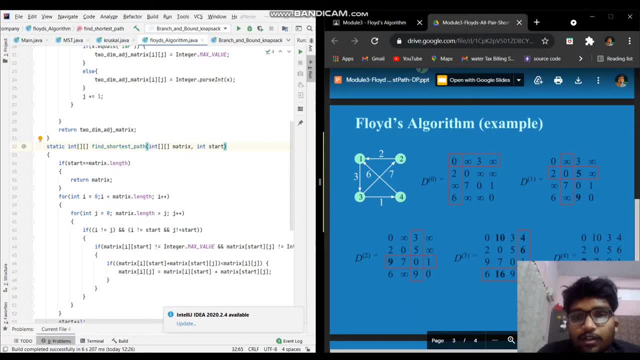 nothing but two to three. so consider going from two to three. so, uh, in the initial cost matrix we have infinity in the place of two to three, because there is no direct edge between two to three, right? so in that case we have given infinity there, but, uh, using uh in the first iteration, we have, uh, what, what we, what we're going to do is. 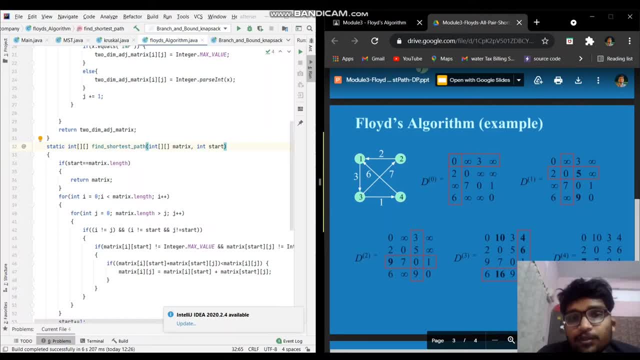 uh, we'll consider one, as we have selected one, right? so if you go from two to three via one, then, uh, the cost would be five, right? so if you go from two to one, the cost would be two, and there, from one to three, the cost would be three. its total would be five. so if you go from two to 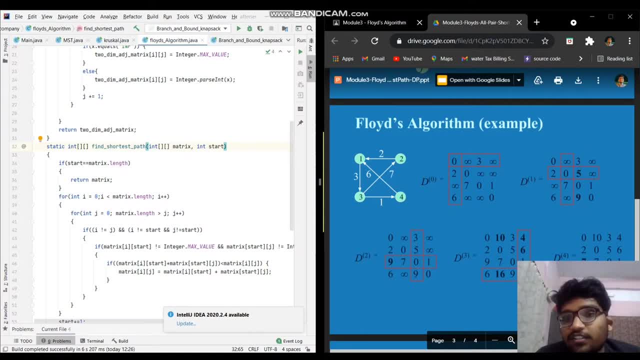 three uh via one, so the cost will be five, right? so in the next uh, in the next iteration, the cost matrix would be updated as five. so in that case, uh, we'll select each row and column in each iteration. so in the first case we have selected. on the first. 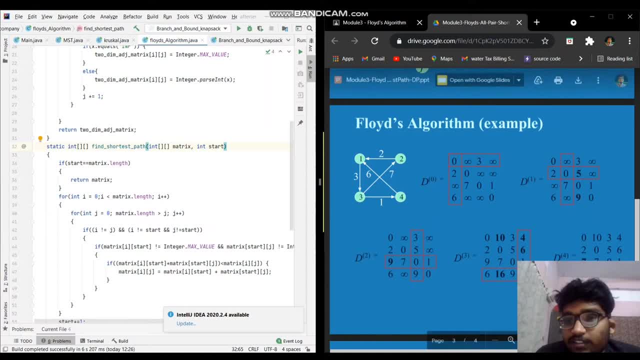 row and first column. in second case we have select, we're going to select second row and second column. so likewise, uh uh, we can see here: if start equals to matrix dot length, so fine. if the if start initially, the start is zero, that means the row and row and column selected is zero, that is one. 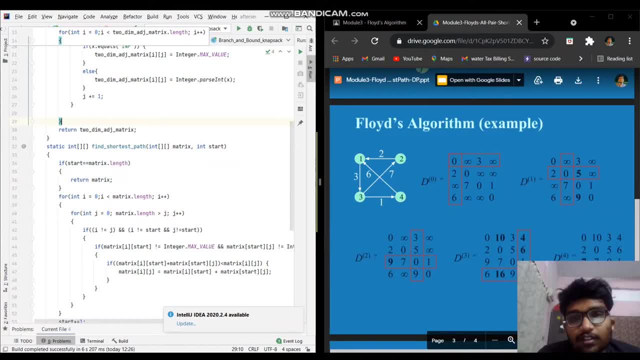 first row and first column. so if the stat is uh equals to matrix dot length, matrix uh dot length would be four here, right? so if all the four rows and columns are selected, then uh would be, start would be four and that would be equal to matrix dot length and our function would: 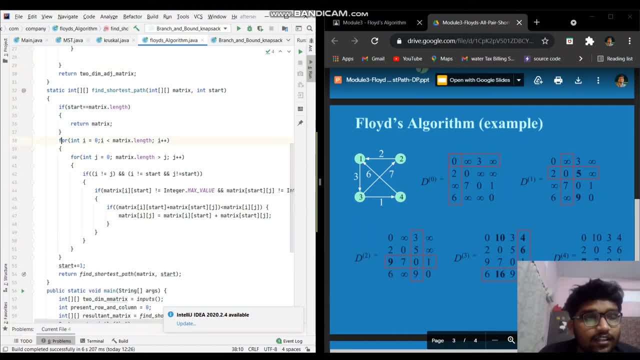 be finished. then after that we have a loop in as else part for this function and uh, we can see here, if i is not equals to j, that means that. uh, if i is equals to j, that indicates a diagonal. so, uh, we do. uh, that diagonal is always zero in the cosmetic side. so we have that condition and i not equals. 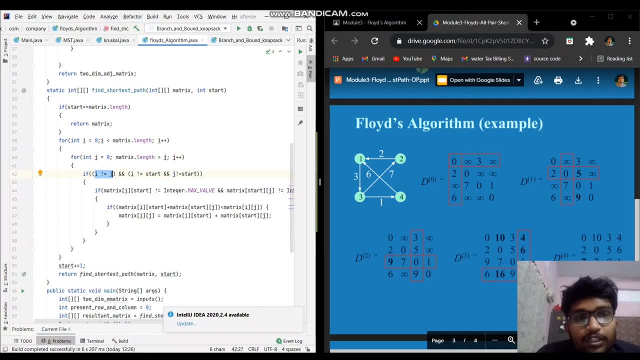 to start and j not equals to stack. so we have uh past zero to the start rate. so if you consider zero, uh, i and j as zero and zero, sorry, zero, sorry, zero and one, so i is not equals to start. but uh, sorry, i is not equal to start would be false and j is not equal to start would be true. so in 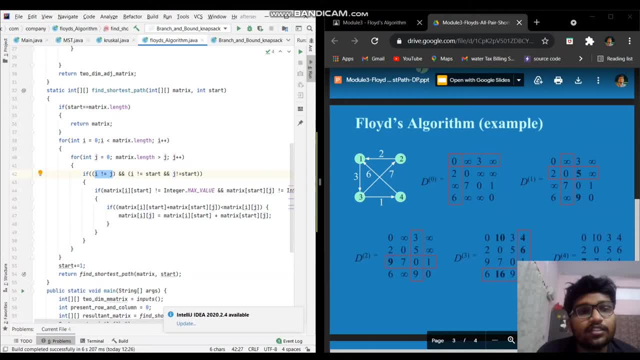 that case, uh, this, uh this, the inner, inner statements will not be executed because, uh, we, we need to neglect that entire row and entire column. so, uh, we need, uh we have, this condition: i not equals to start and j not equals to start, and after that we have, if matrix of i and 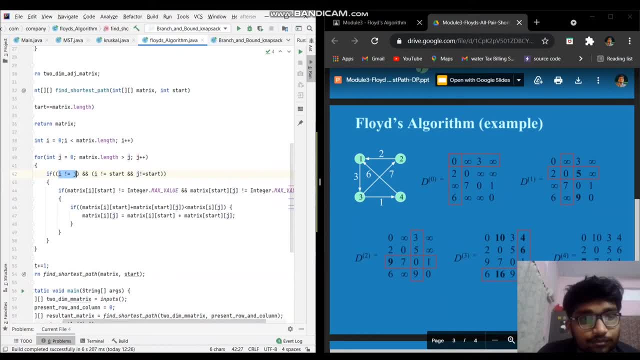 j is not equal to integer root max value. that means that if, if the particular cell is not equals to integer root max value, that means that infinity consider it as infinity. only then we are going to update that because inside the statements we can see that if matrix of i and start and plus 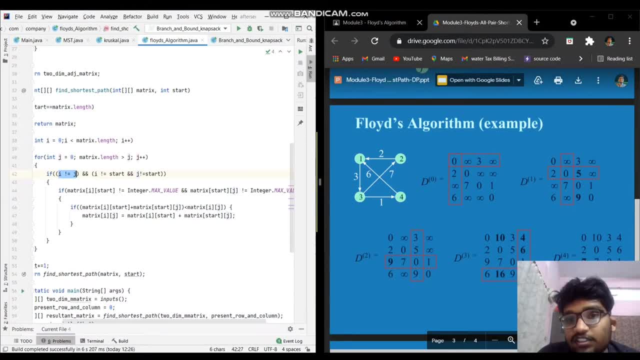 matrix of star engine. that means that if you go from uh, for example- consider this case- if you go from two to three via one, if the cost is less than the current entry- i mean current entry is infinity, the infinity- then we would update that entry. so here 5 would be less than infinity, right? so 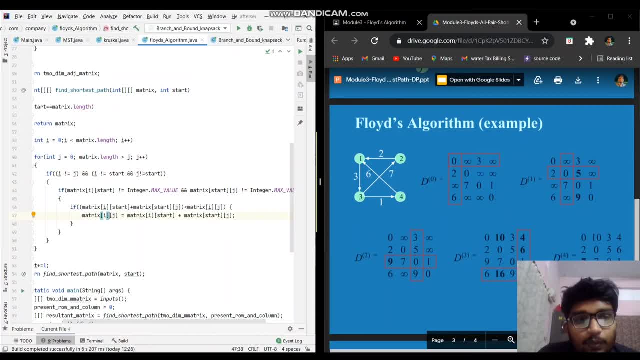 in that case the matrix, that particular entry, will be updated. otherwise we will not update that. but if any of these, for example if any of these operands is infinity, that is, integer dot max value, then obviously that would not be less than any of this value, right? so in that case we will. 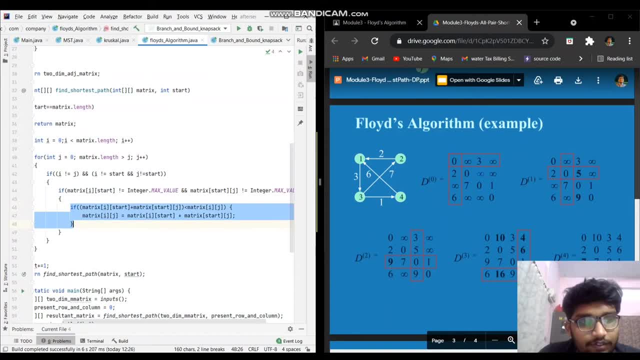 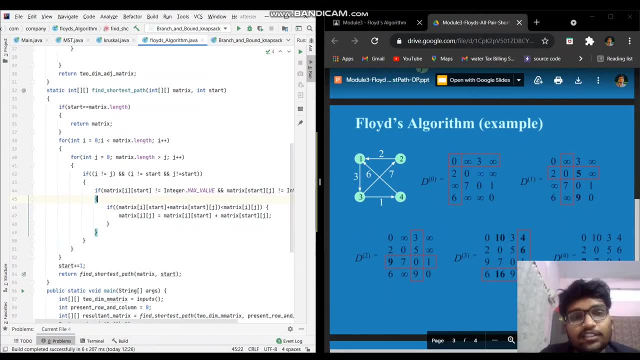 not, we are not going to consider this if statement so fine. that's why we are going. we are checking this if statement in the previous. if fine, then after that we are incrementing the start by one. that means selecting the next row and column and we are calling the function same function. 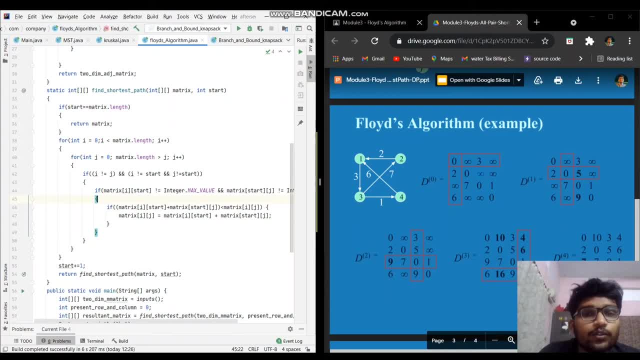 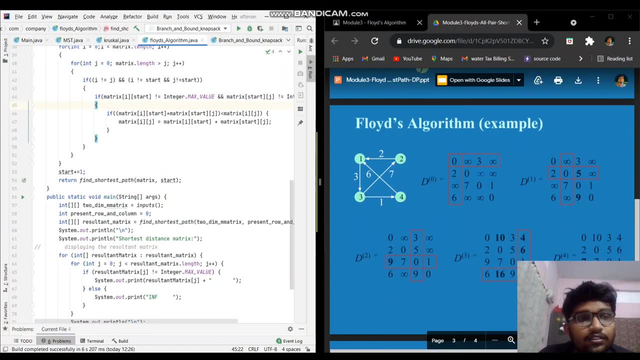 recursive function with the same matrix and the incremented start value. so in that way we are going to find the shortest possible path between all the pairs of vertices and we are going to return that here. we can see, this is the base condition. we here, we are returning the cost. 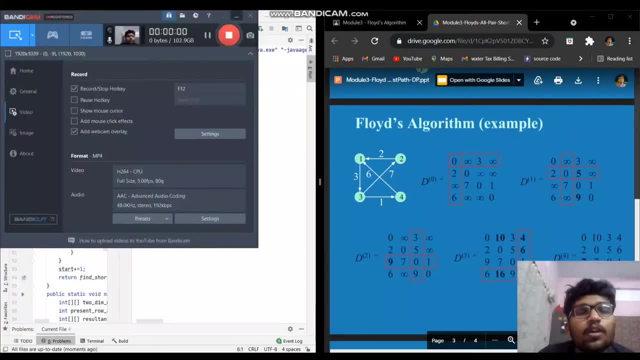 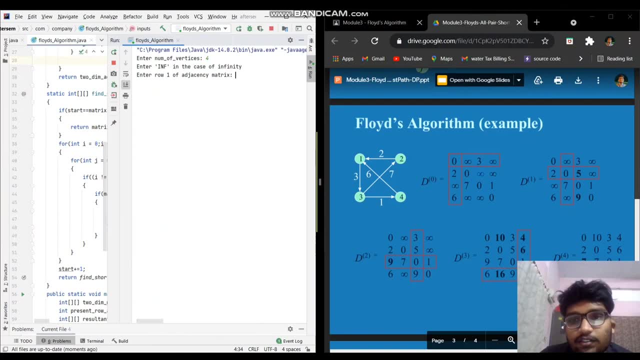 matrix. fine, after that we are going to print this. now let us run this code and check for this same input. so render number of vertices would be 4 and row 1, that is, 0, infinity 3 and infinity right. so 0, inf, 3 and inf. in the second row is 2: 0, inf and inf and inf. 7, 0, 1 is the third row: 6, inf, inf and. 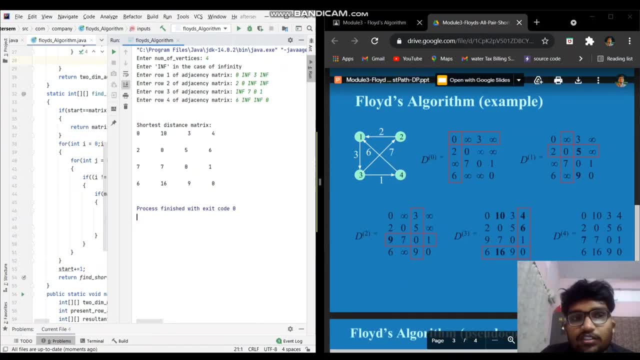 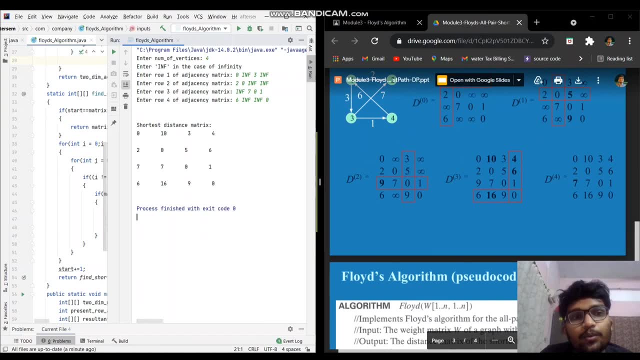 0 would be the fourth row. yes, we can see. the shortest distance matrix would be this one: 0, 10, 2, 0, 5, 6, 7, 7, 0, 1, 6, 16, 9 and 0. I hope the output value is correct and thanks for watching.